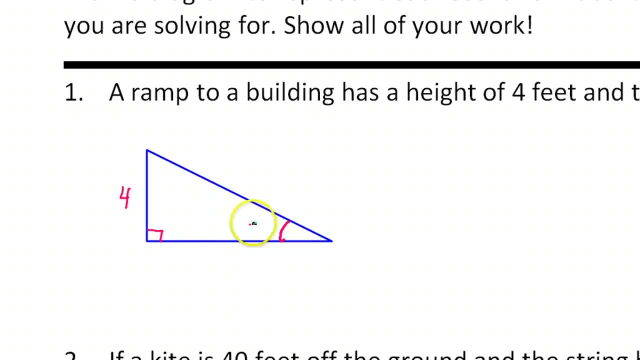 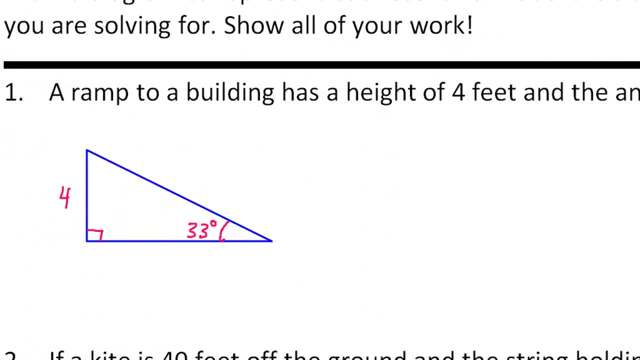 to the ground. so that means that this is 33 degrees. And see how long is the ramp. Okay, so the length of the ramp is the hypotenuse here, because this is the ramp is really the hypotenuse. Okay so how long is the ramp? So let's just call that x. 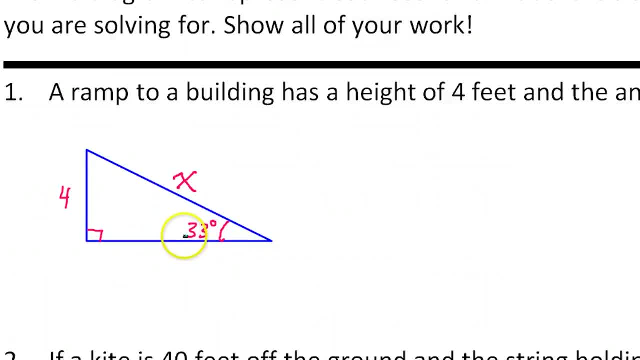 So the key to solving these ramps, real-world problems, is to draw the picture correctly. Once you have that, then it's just a normal problem. So you know, we decide which trig function are we going to use. And from the 33, the 4 is opposite. okay, because it's a cross from and, of course, 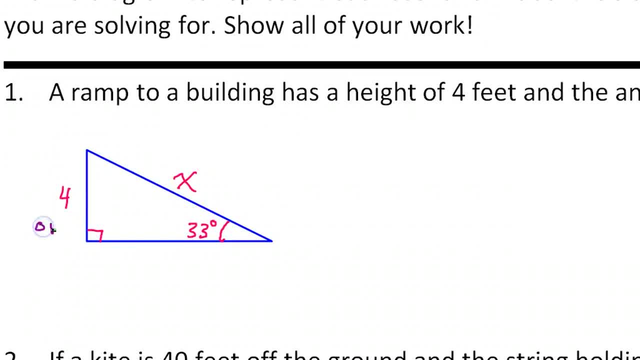 this is the hypotenuse. So you know we've got opposite and hypotenuse. So which trig function is it? So we've got the trig function and we've got the hypotenuse, So which trig function? 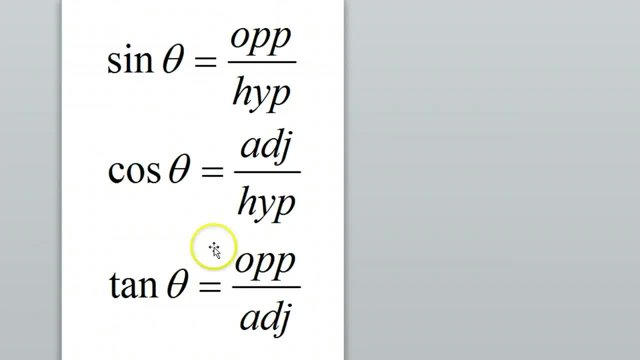 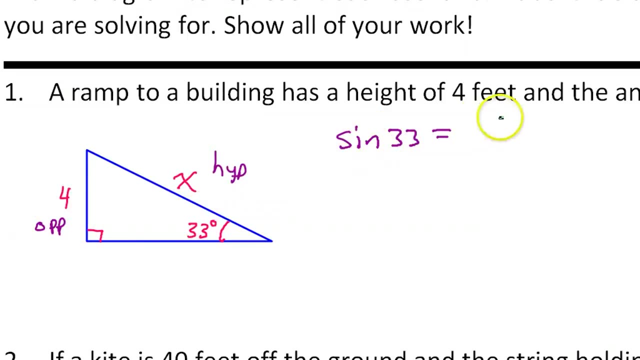 is it? So we've got the trig function and we've got the hypotenuse. So which trig function is that? well, that's the sine function is the sine of the angle is opposite over hypotenuse. so that means that the sine of 33 degrees is equal to opposite over. 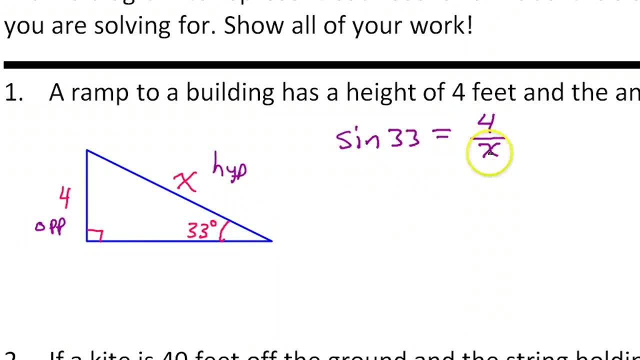 hypotenuse, so that's 4 over X, all right. now, when the variable is in the denominator, it's a useful to do this shortcut, because the denominator and the quantity by itself can be reversed all right. it's just a little shortcut that comes up often enough that it's worth just memorizing, so that would make this. 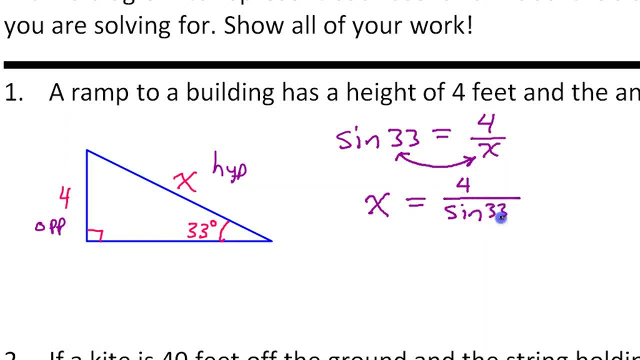 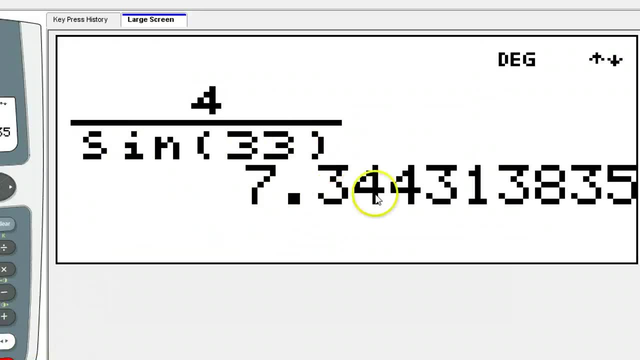 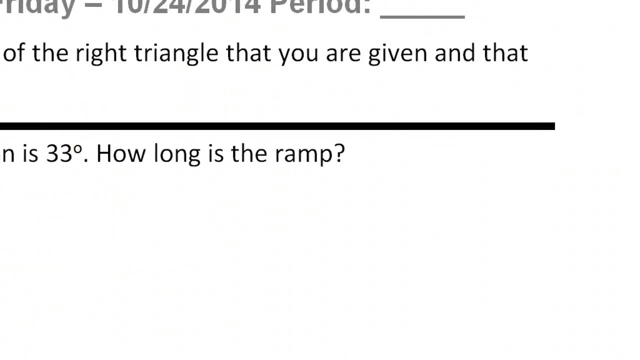 X here and the sine 33 would come here. okay, and I would just put this into the calculator and that's going to give you the length of the ramp. in your calculator it would look like that. so we get 7.3. blah, blah, blah. let's see were we told to what? how? 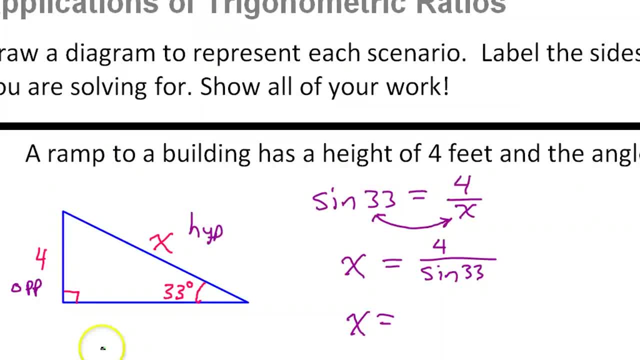 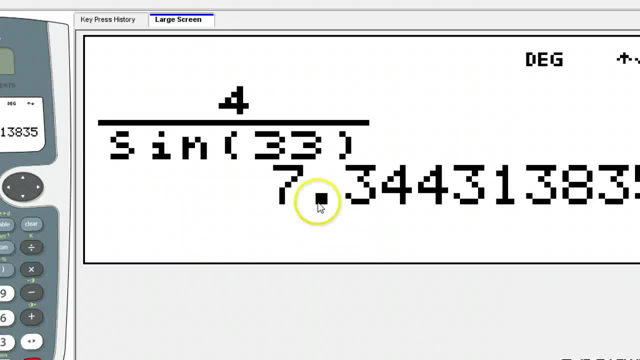 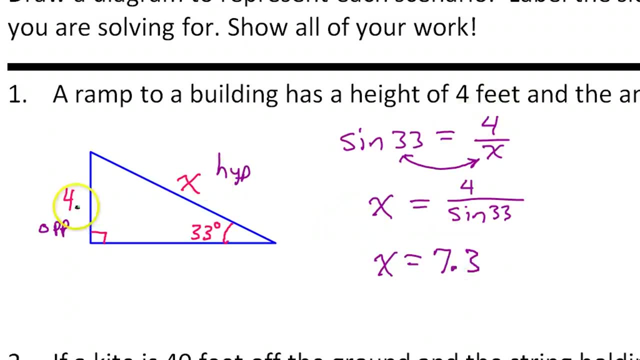 many decimal places. all right, it didn't say how many decimal places, so let's go ahead and do one decimal place. okay, so let's call it 7.3. and we're talking about feet. I should have put that right there as well: 7.3. 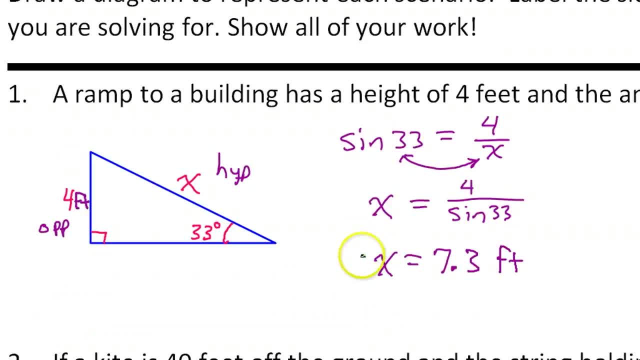 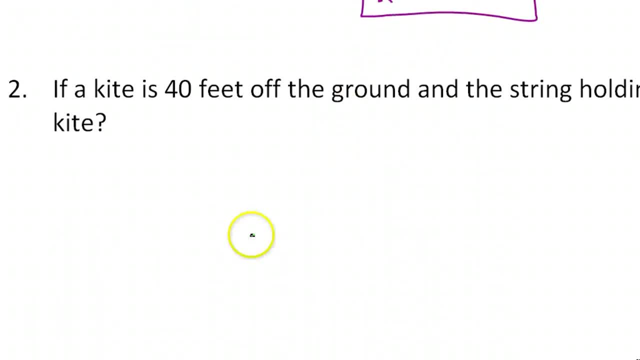 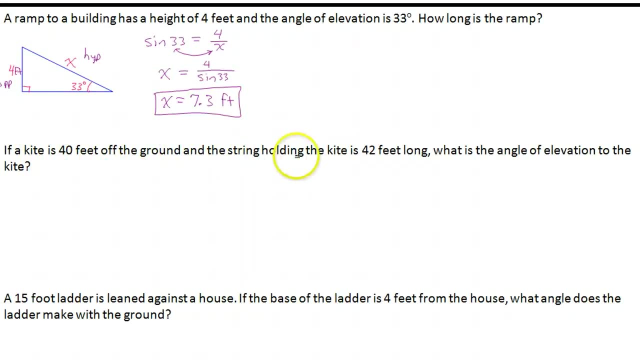 feet. okay, and that is how long that ramp is. all right, let's go ahead and take a look at number two. okay, if a kite is 40 feet off the ground and the string holding the kite is 42 feet long, what is the angle of elevation to the kite? 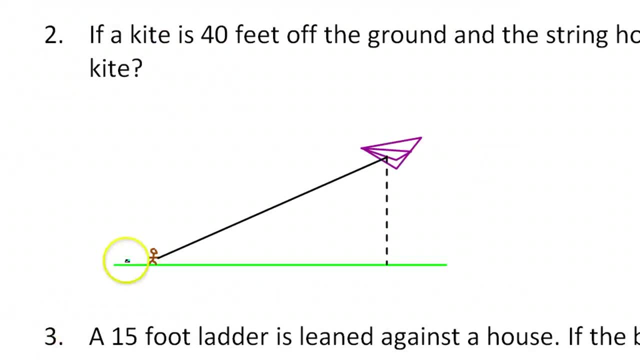 okay, if a kite is 40 feet off the ground and the string holding the kite is 42 feet long, what is the angle of elevation to the kite? all right, let's draw that picture, okay. so here's the situation: the kite is 40 feet off the ground, so that means this height right here is 40 feet. okay, and 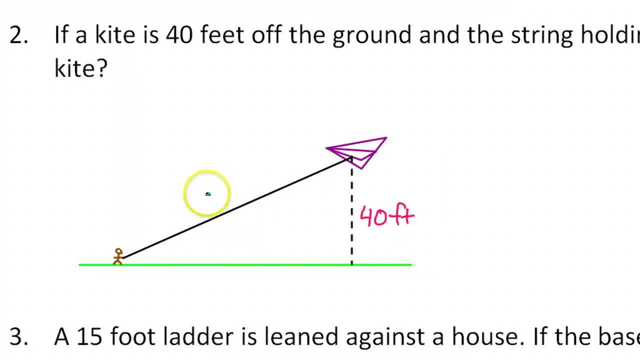 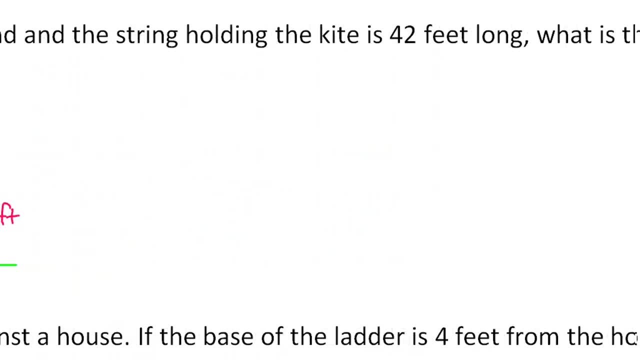 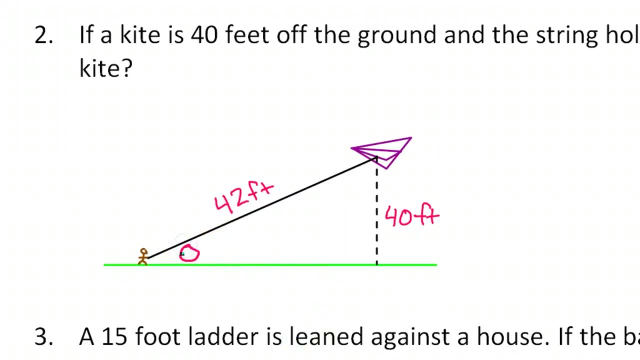 the string holding the kite is 42 feet long. so the string here is 42 feet long. okay, what is the angle of elevation to the kite? all right, so the angle of elevation is the angle to the ground. so this would be the angle of elevation. all right, how do we find angles, guys? inverse trig functions all. 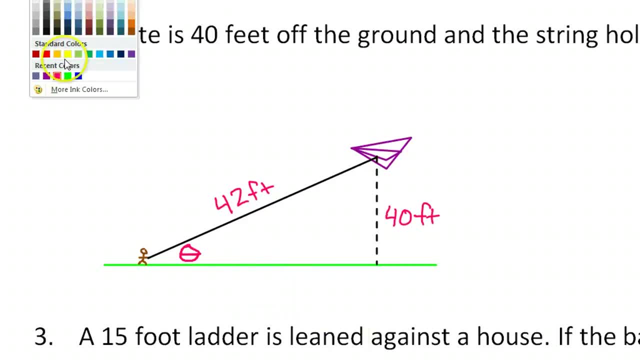 right. so first you have to pick which trig function you're actually going to use and from the angle of elevation, here this is opposite. all right, because it's across from it, and of course this is the hypotenuse, no matter what. so we have a totally opposite angle. all right, sausages, Arena, Juliet. all right, and 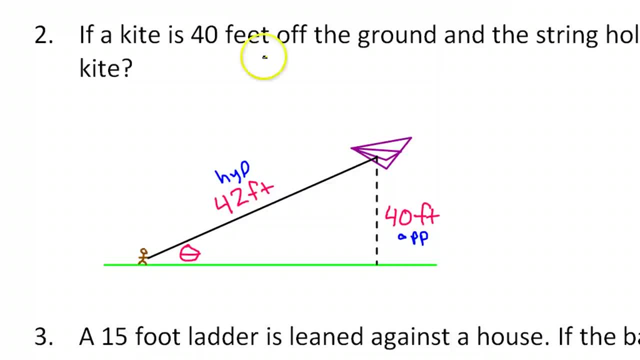 the squared side is 0, you go, I'm going to. alright, so this is theline. so what we're saying of theta? right, we would find angle dash, jor and theta in one direction, that's an angle in the inverse sign of 40 over 42, and then we can just put this in our calculator. 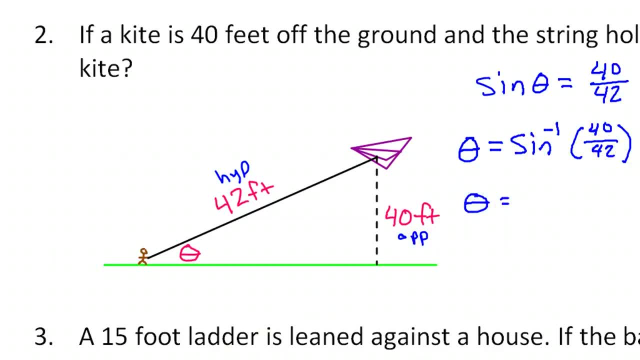 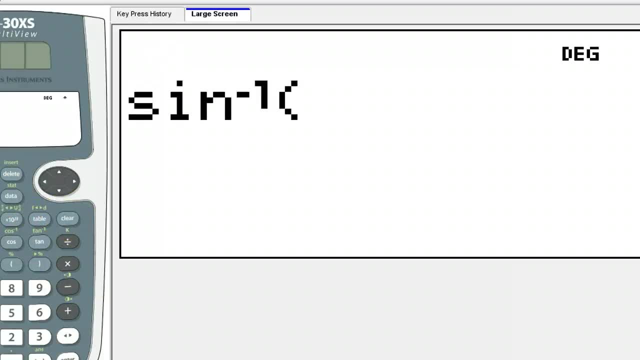 to find out what the angle is. so inverse sine of 40 over 42 would look like this: well, let's clear this out. so you have to hit second sine of 40 over 42. all right, and to one decimal place, that's 72.2. 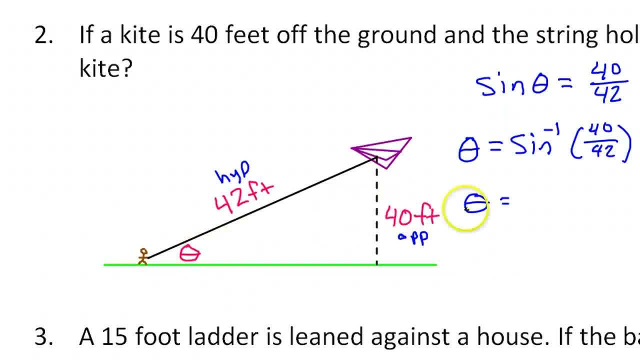 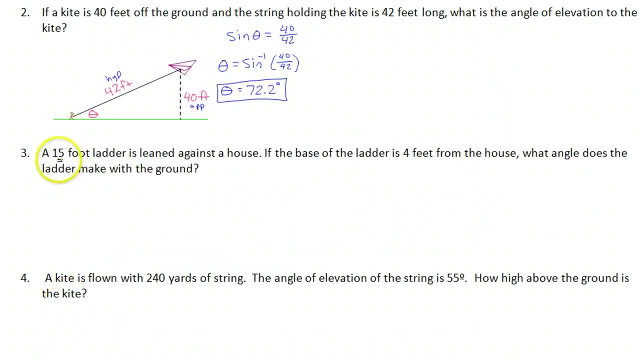 degrees, all right. this is an angle, all right. so 72.2 degrees, all right. so that will be the answer to number two, all right. number three: a 15 foot ladder is leaned against a house. you can see that the ladder is leaned against a house. 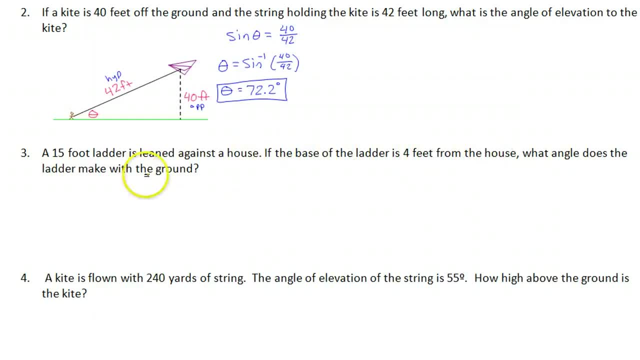 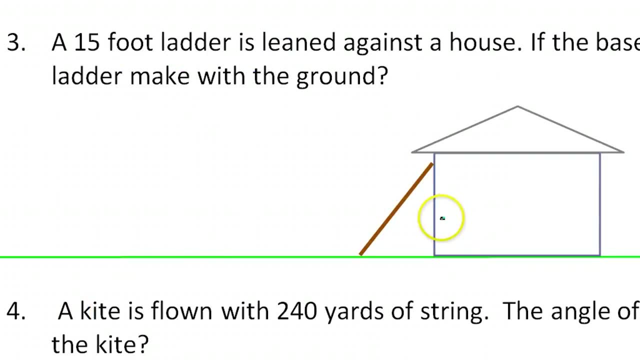 so that's the answer to number two. all right, so that will be the answer to number two. If the base of the ladder is four feet from the house, what angle does the ladder make with the ground? Okay, so this is a ladder leaning against the side of this house. 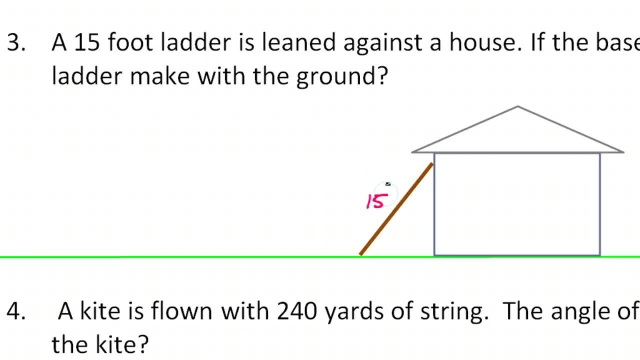 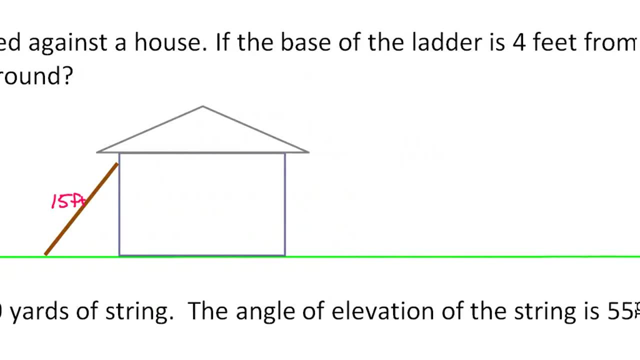 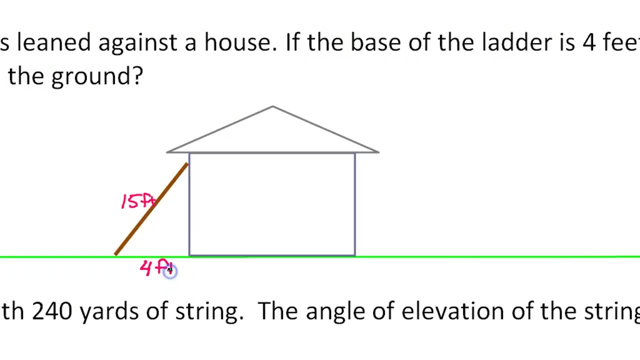 It is a 15-foot ladder. Okay, so 15 feet. We'll go right there, leaning against the side of the house. The base of the ladder is four feet from the house, So that means this is four feet right here. 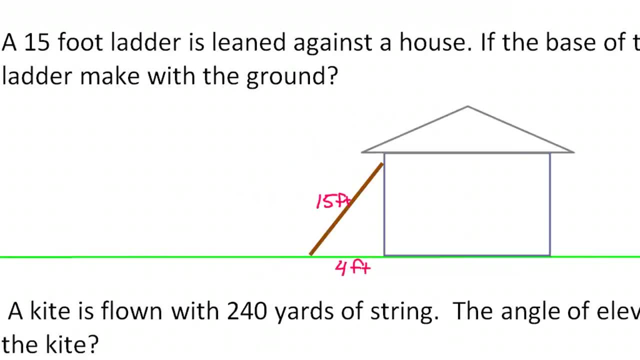 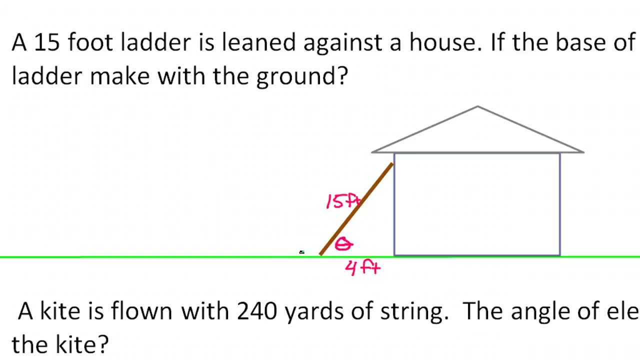 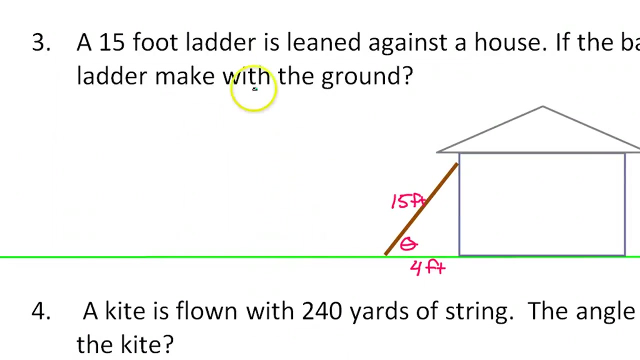 And we want to know: what angle does the ladder make with the ground? Alright, and that's just like the angle of elevation, Okay. so again, if you want to find the angle, how do you find the angle? You find angles using inverse trig functions. so that's what we're going to do. 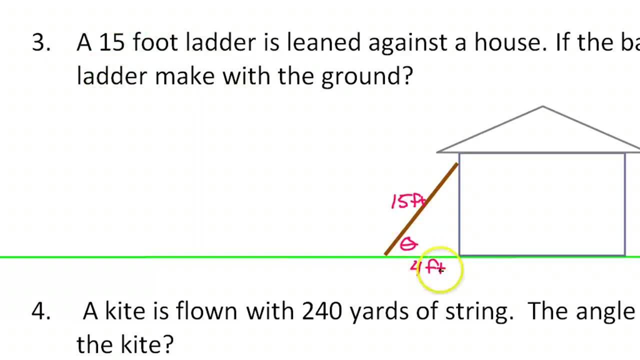 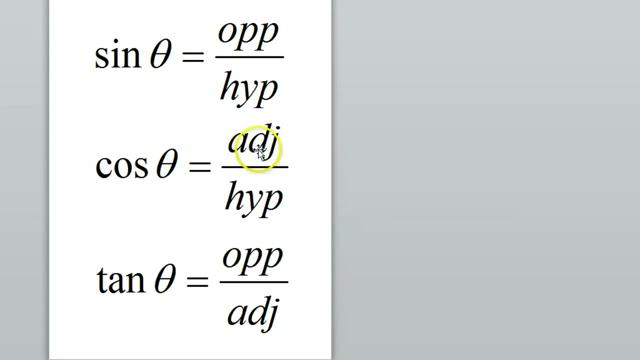 But first we need to decide which function we're going to use. Well, from the perspective of this angle, this four feet is adjacent And of course the ladder here is the hypotenuse. So, adjacent and hypotenuse, hmm, why? that's the cosine function. 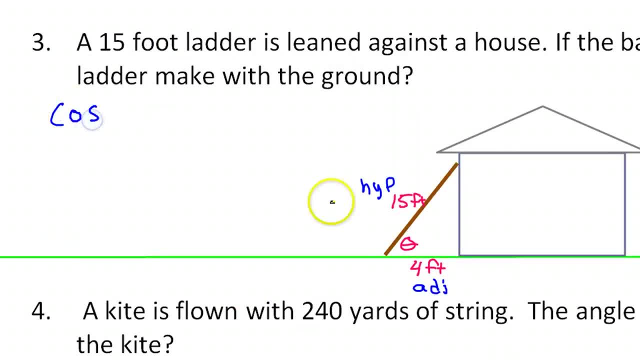 So I will start off using the cosine function. So I will say the cosine of the angle is adjacent over hypotenuse, So that is four over 15.. But like I said, If you want the angle you must use the inverse trig function. 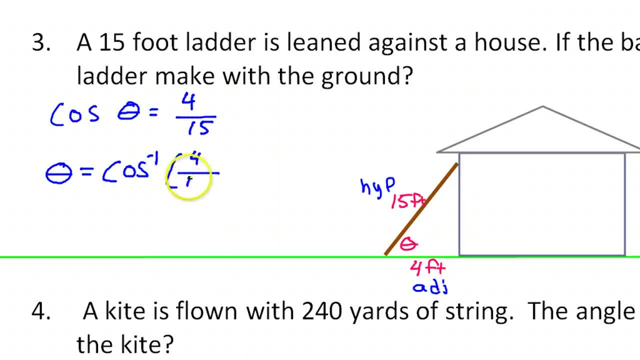 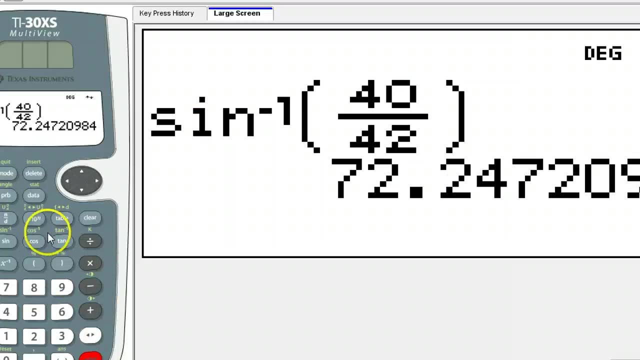 So that will be the inverse cosine of four over 15.. And you can just put that in your calculator and that will give you the actual angle, Inverse cosine four over 15.. Whoops, I didn't need that. Okay, so second cosine does it, and four over 15.. 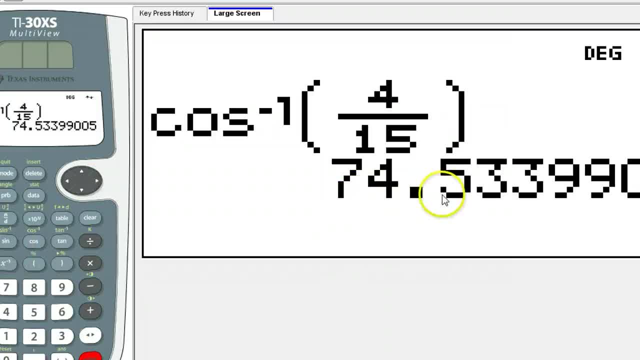 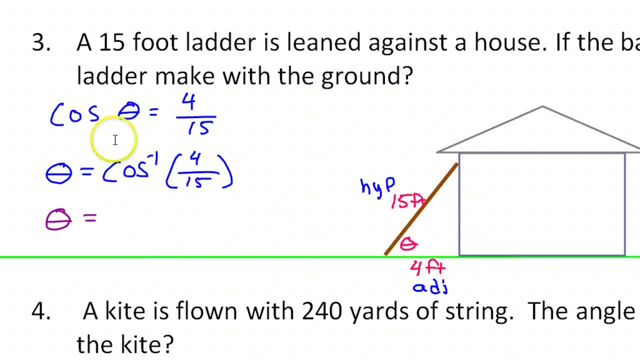 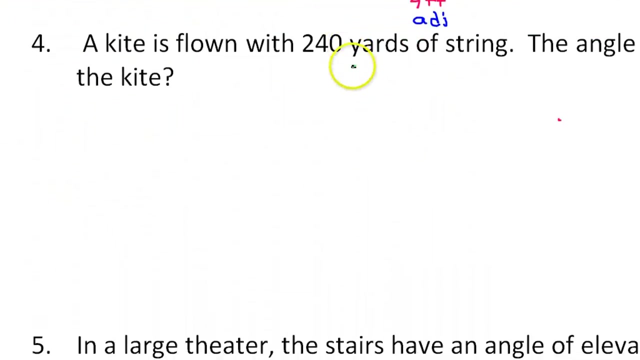 Okay, so that's 74.5 degrees. alright, this is an angle, So that is 74.5 degrees. Okay, that would be how big the angle is. Alright, How about number four? A kite is flown with 240 yards of string. 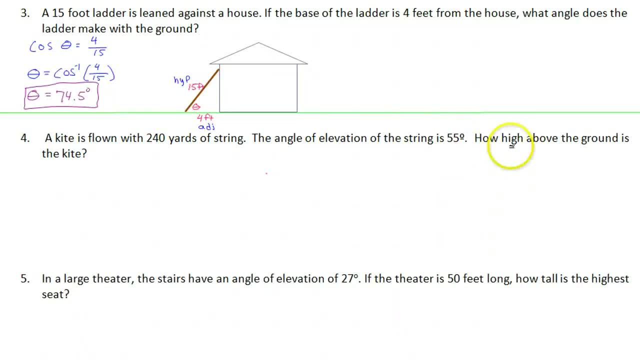 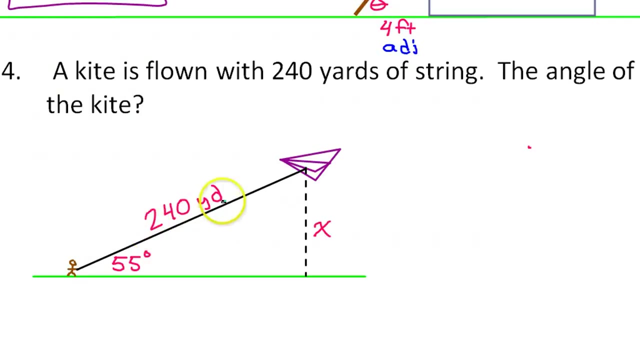 The angle of elevation of the string is 55 degrees. How high above the ground is the kite Interesting? I'm just going to cut and paste my kite picture from before. Alright, so here's the situation: A kite is flown with 240 yards of string. 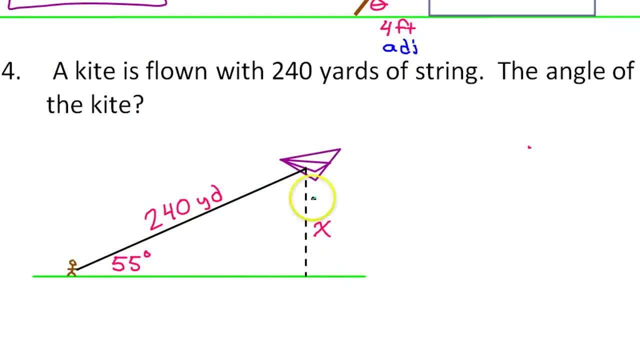 Angle of elevation is 55 degrees And we want to know how high off the ground is the kite. So that would be x, right here, Okay. well, from the perspective of this angle, our unknown over here is the. this is opposite. 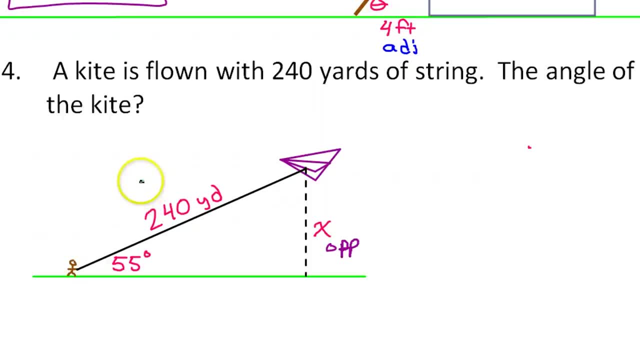 Because it's across from the angle. Of course, the 240 is the hypotenuse, no matter what. So which trig function involves opposite and hypotenuse? By the way, you should have this memorized by now. That is the sine function: opposite over hypotenuse. 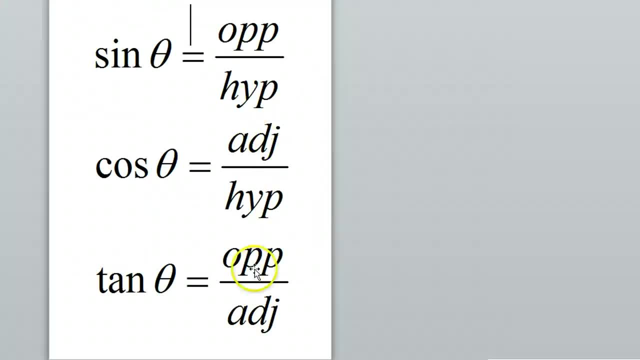 Okay, Yeah, if you haven't memorized these yet, stop and memorize them right now. You know what I mean Like study this chart and then look away and go try to write these down on another piece of paper And then look back and see if you were right. 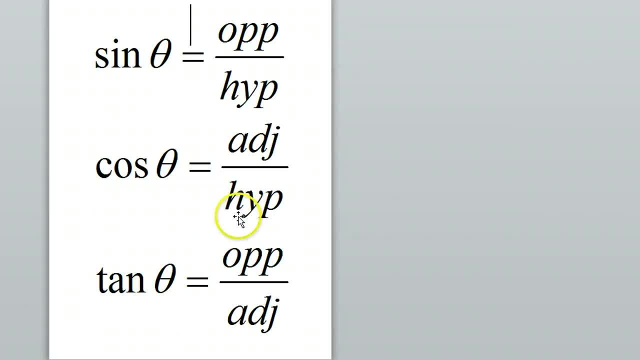 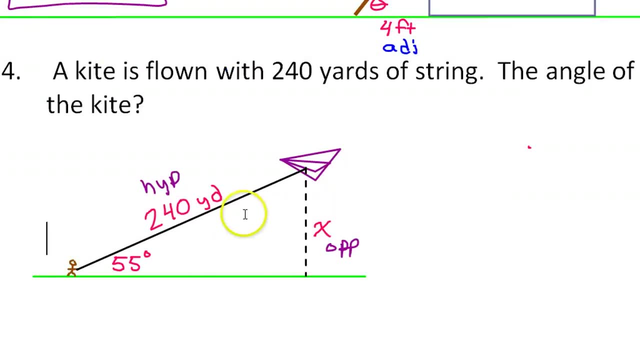 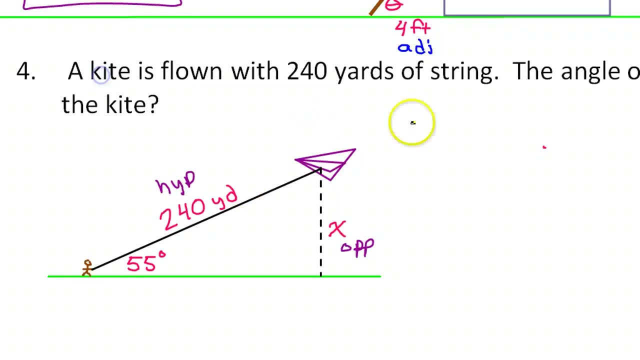 And do that over and over again until you can get it every single time. Alright, It's called studying, And that's what that sounds like. I'm sorry, that was a little sarcastic. So the sine function is what we're going to do. 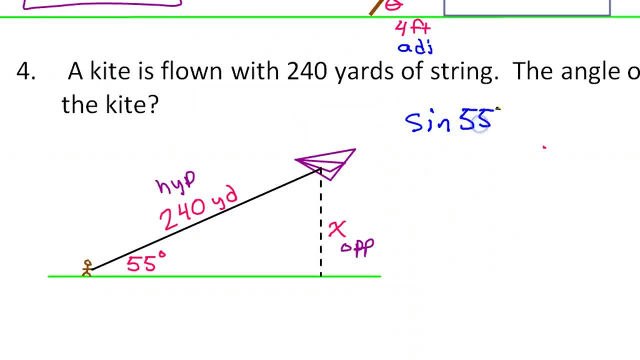 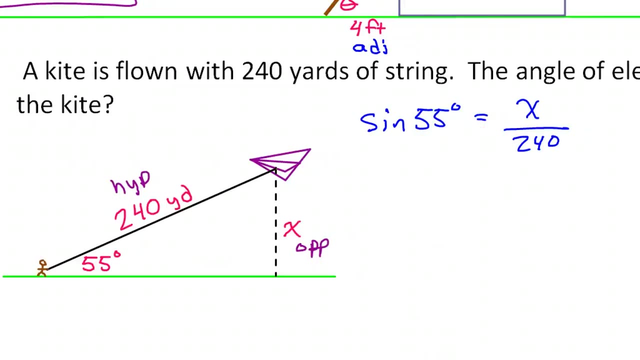 So the sine of 55 degrees is opposite over hypotenuse, So that would be x over 240.. Okay, this dot is bothering my OCD. Um, To solve this, do I need to do the swap thing? Uh, no. 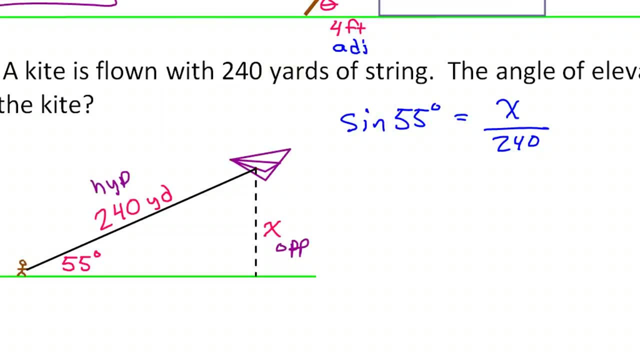 That only helps me when the variable is in the denominator. Instead, I should multiply both sides by 240.. Alright, That way these will cancel out. Okay, So that's going to just leave me with. you know, 240 sine 55 is equal to x. 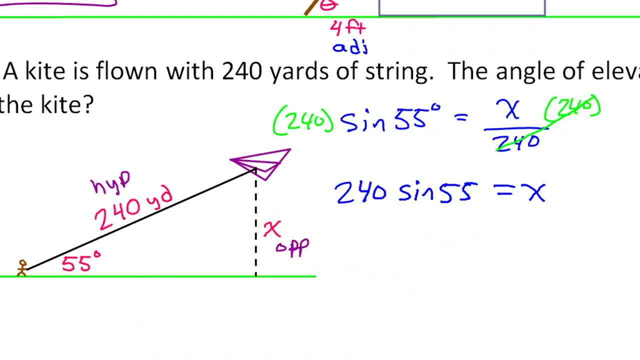 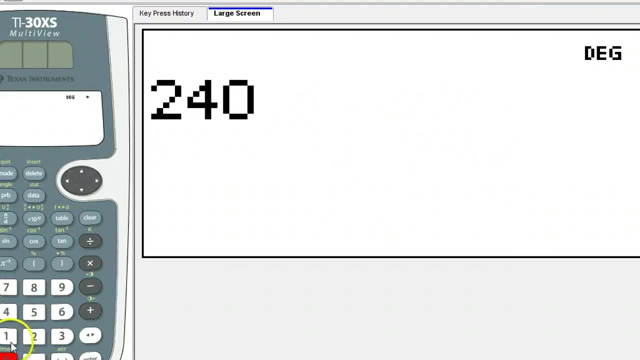 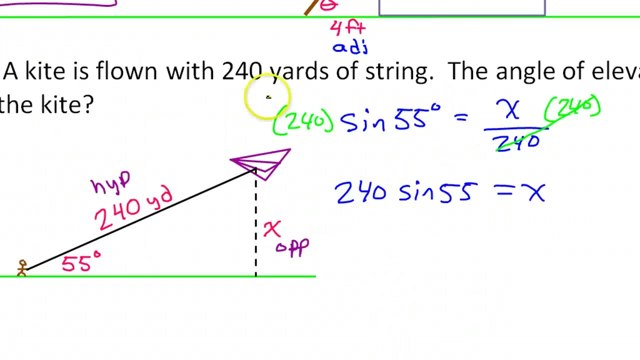 And you can just put this in your calculator: 240 sine 55.. Okay, 240 sine 55.. Alright, So that is 196.6.. Gotta round up 196.6.. Okay, 196.6 yards. 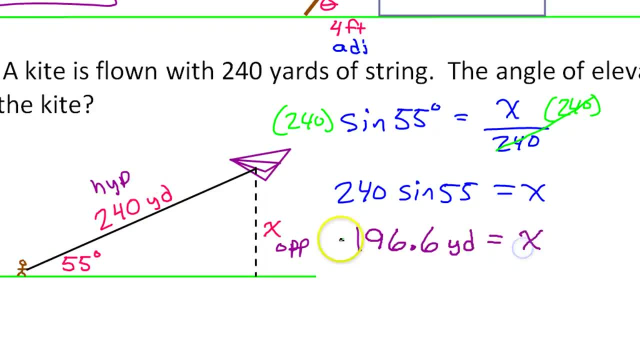 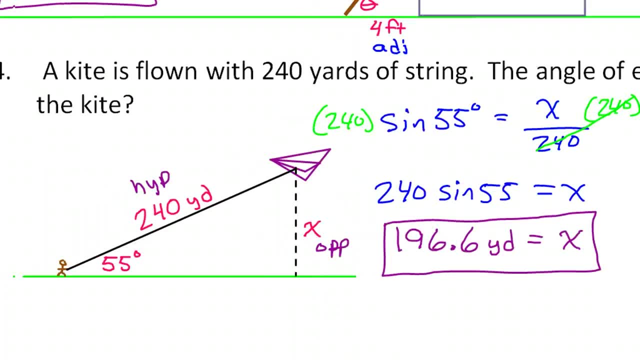 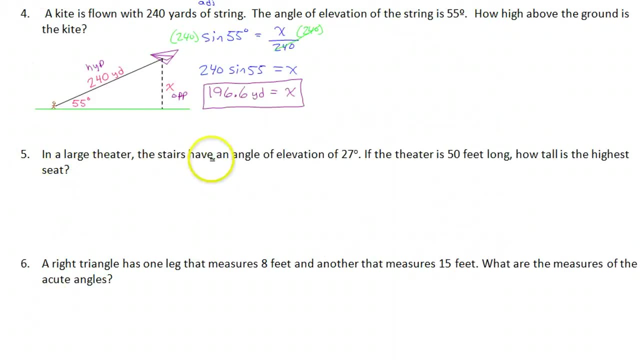 Alright, When you're doing a word problem, a real world problem, the units are very important, So do not leave off your units. Okay, But that would be the answer to number four. Alright, In a large theater, the stairs have an angle of elevation of 100,, I'm sorry, angle of. 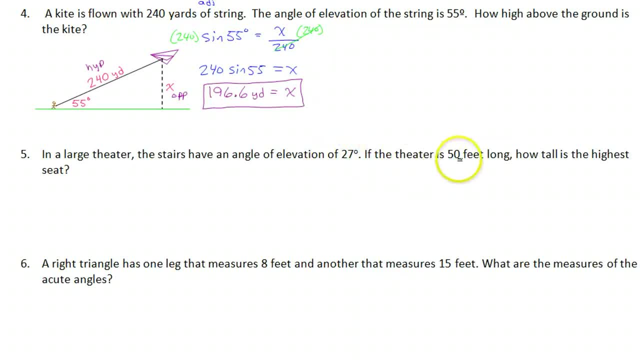 elevation of 27 degrees. 27 degrees. If the theater is 50 feet long, how tall is the highest seat? Okay, Well, I don't have any clever way of drawing stairs, Um, so I'm just going to draw a triangle. 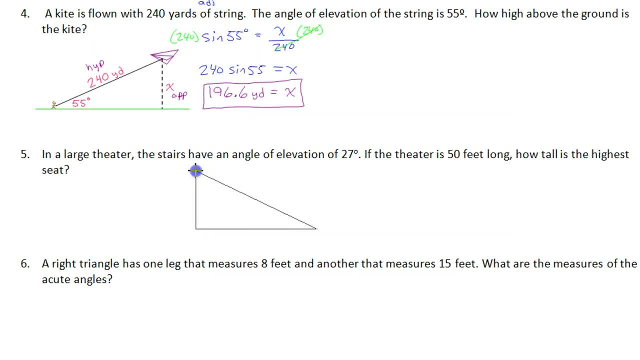 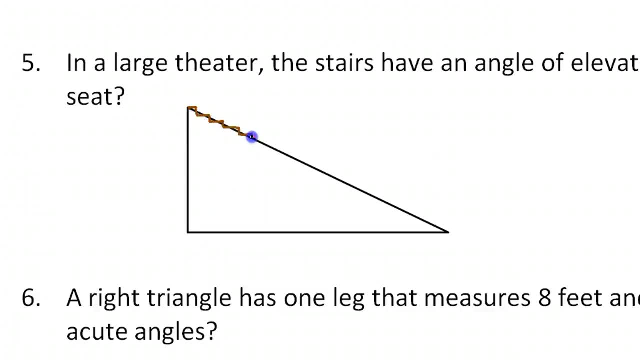 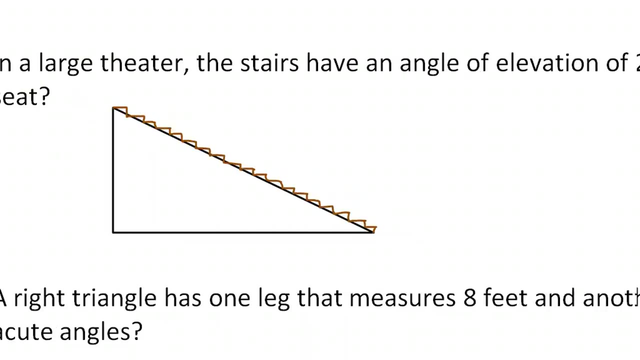 Alright To represent my stairs in this theater? Okay, But just understand. alright, in this picture the stairs are like here: Alright, Okay, I'm messing that up, but you get the idea. Alright, They say the angle of elevation is 27 degrees. 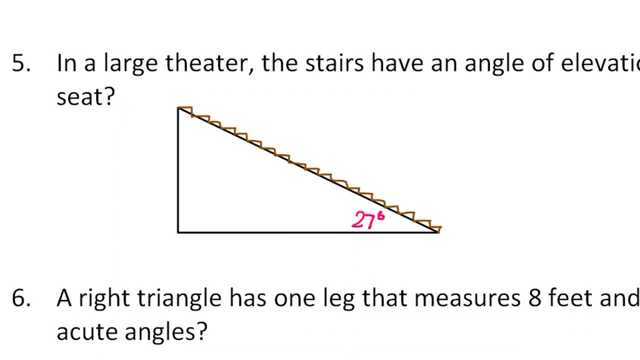 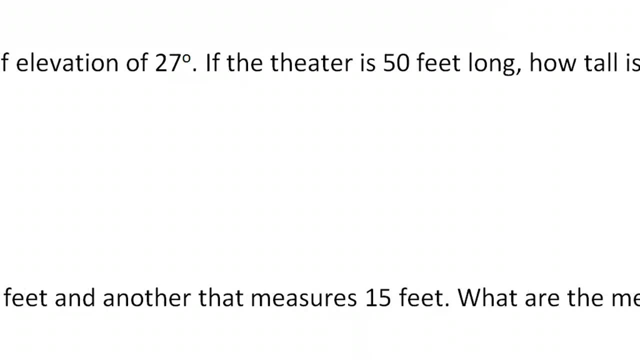 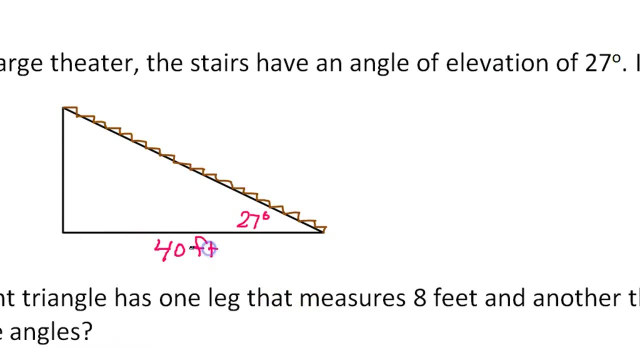 Alright, So that's the angle with the ground. It's 27 degrees. Alright, The theater is 40 feet long, Okay, So, uh, I interpret that to be this: Okay, The theater is 40 feet long, Okay. 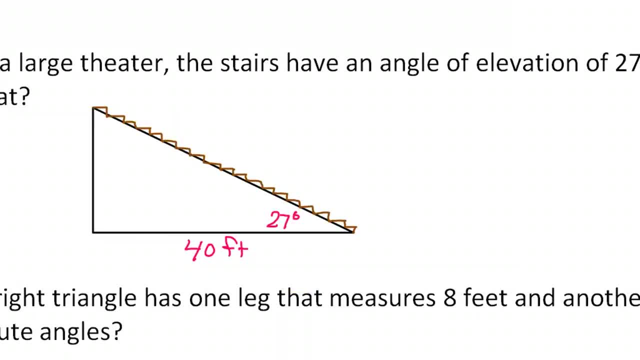 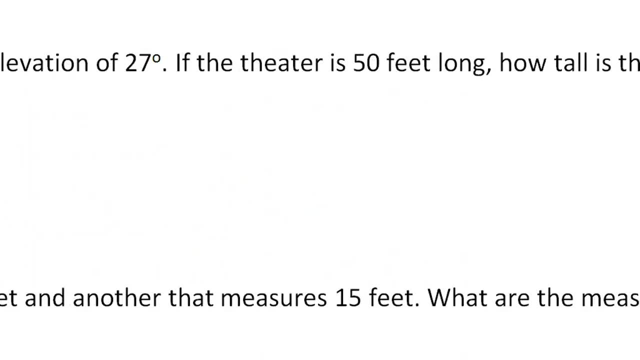 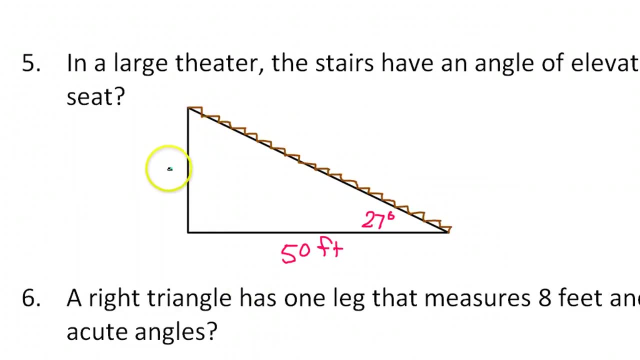 Um, no, 50 feet long. The theater is 50 feet long. I'm a little blind right now, sorry. The theater is 50 feet long. How high is the? um? how tall is the highest seat? So the highest seat is going to be up here, so we're being asked for the height, right? 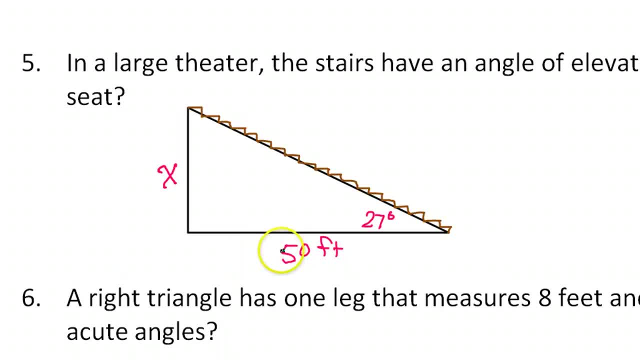 here, Okay, So. So which trig function are we dealing with? From the perspective of the 27 degrees, this height is opposite, It's the opposite leg And, uh, this length of the theater is the adjacent leg. Hmm, 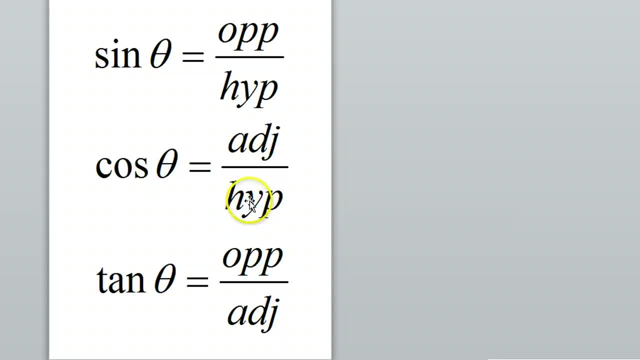 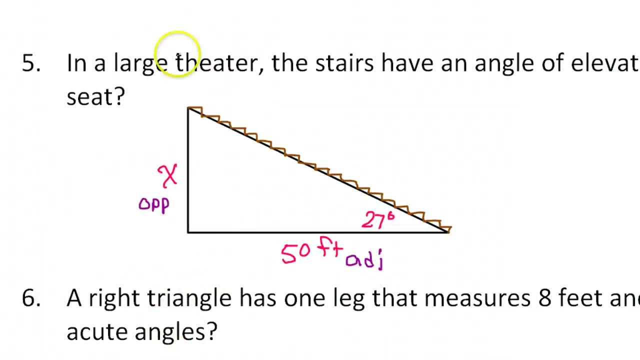 Opposite adjacent. Which function is that? Well, cosine is, wait, no, Strike that Tangent is opposite over adjacent, Opposite over adjacent. So the tangent function. Okay, Um, so we will be using the tangent function. 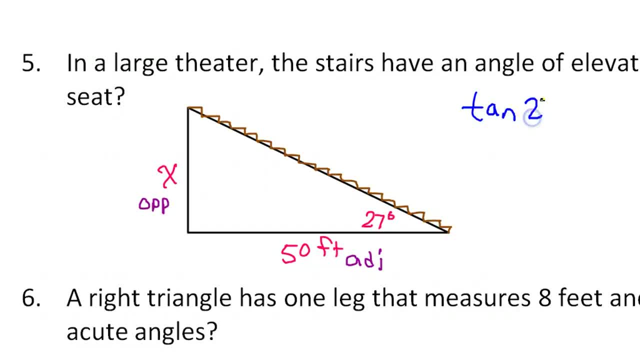 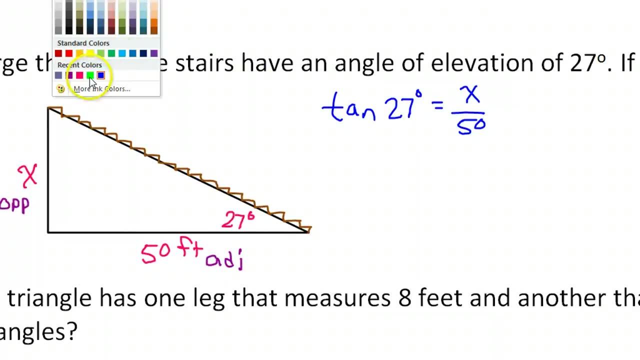 So we will say: the tangent of 27 degrees is equal to opposite over adjacent, So x over 50.. Okay, So to solve this we will simply multiply both sides by 50. And that way these 50s will cancel out. 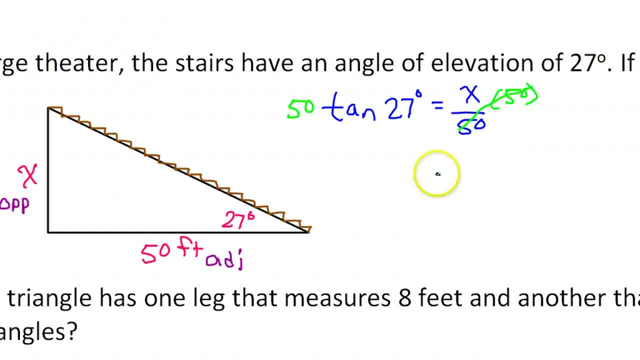 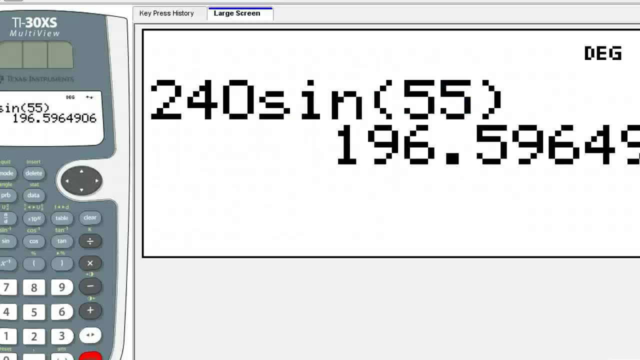 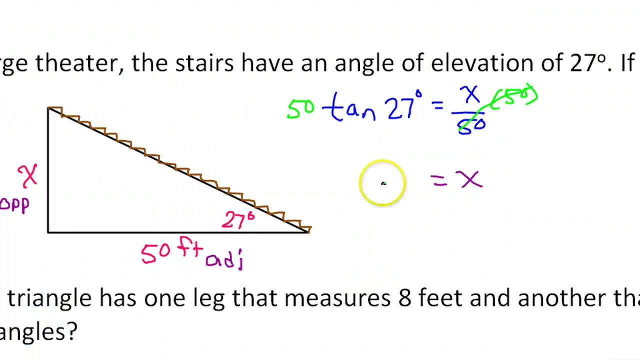 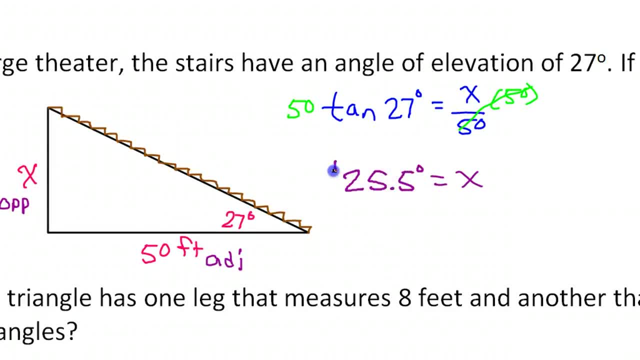 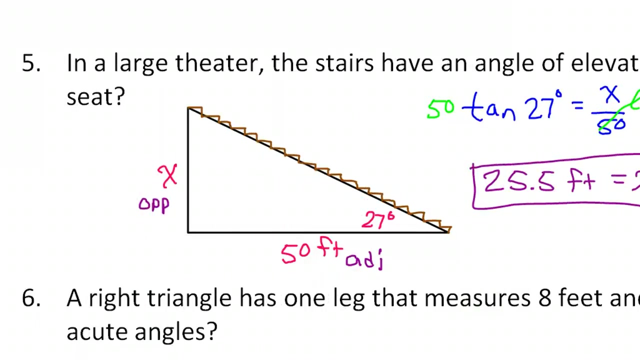 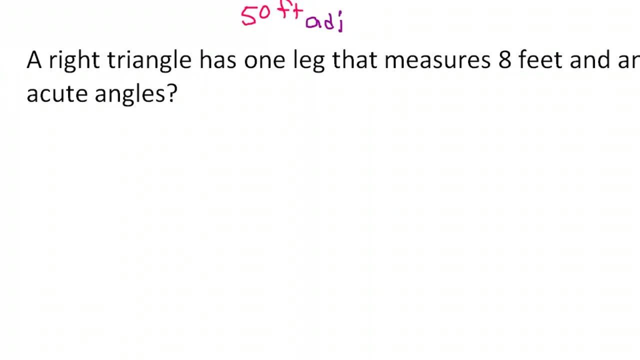 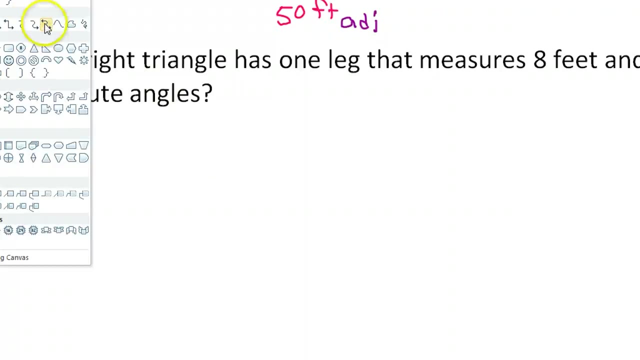 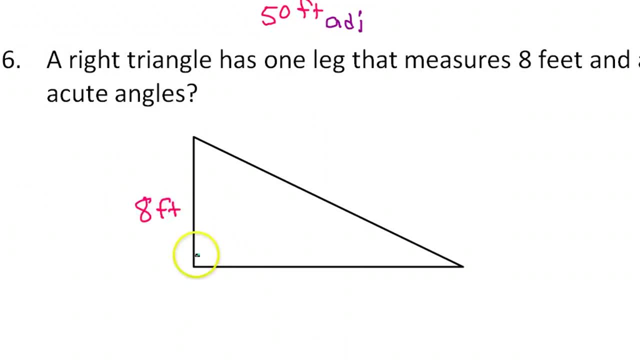 so this will be my 8-foot leg, okay, and this one is 15 feet, and we're supposed to find the measures of the acute angles of this triangle. So how do we find angles? We use inverse trig functions, of course, So just pick an angle, it doesn't matter. So say, if I pick this angle, right? 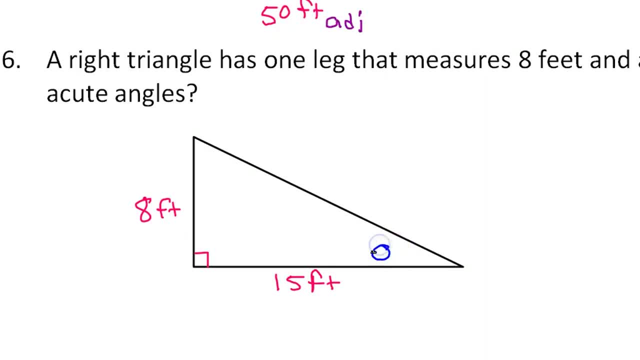 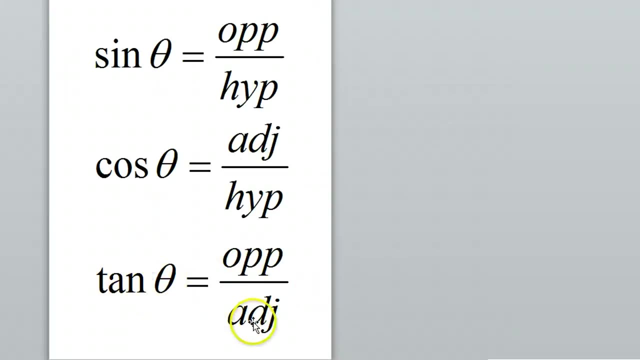 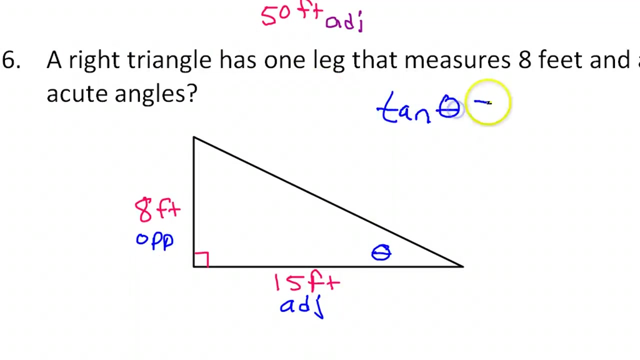 here. okay, I'll just call that theta for right now. Then the tangent: this is opposite and this is adjacent. okay, so that's the tangent function. Tangent of an angle is opposite over adjacent. so that would mean that the tangent of theta is going to equal 8 over 15,. okay, and to find the angle we use the inverse. 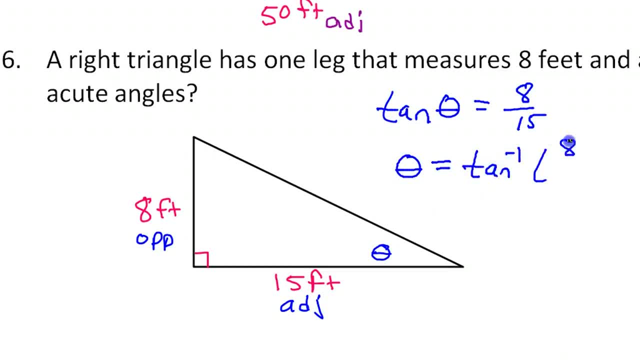 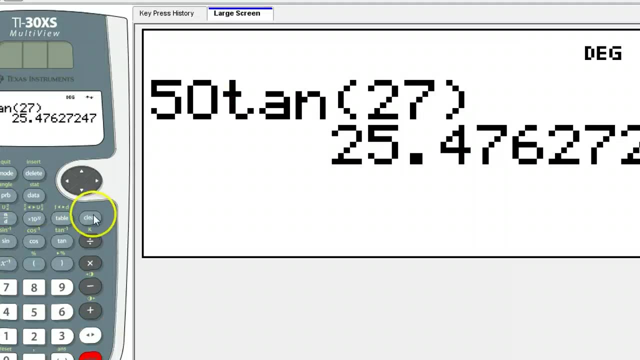 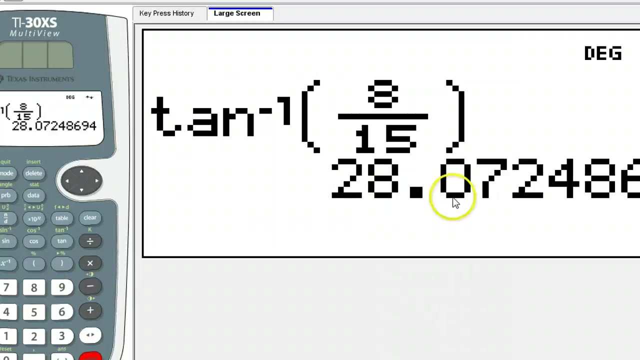 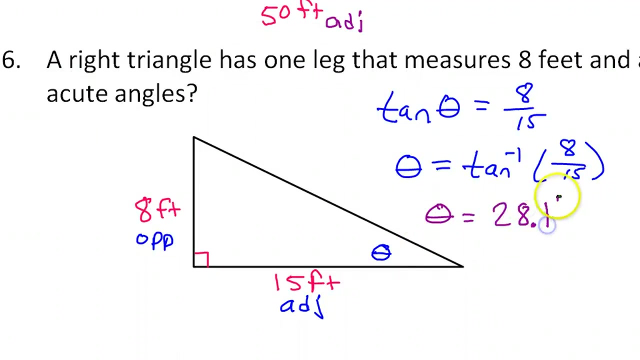 trig function. So that would be inverse tangent of 8 over 15,. all right, so that tells me that theta will equal. whoops, didn't mean to do that. so the inverse tangent. so I will do second tangent of 8 over 15,. okay, is that right? Yeah, So that's going to be 28.1,. got to round up degrees 28.1. 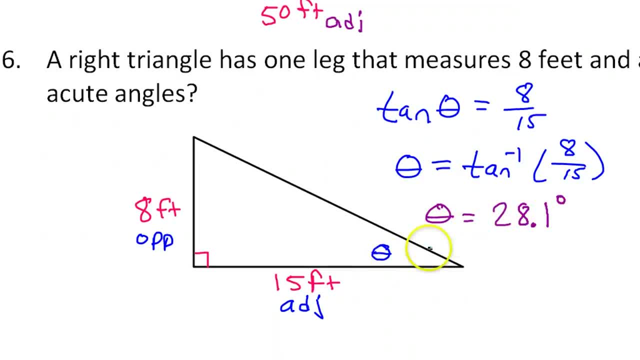 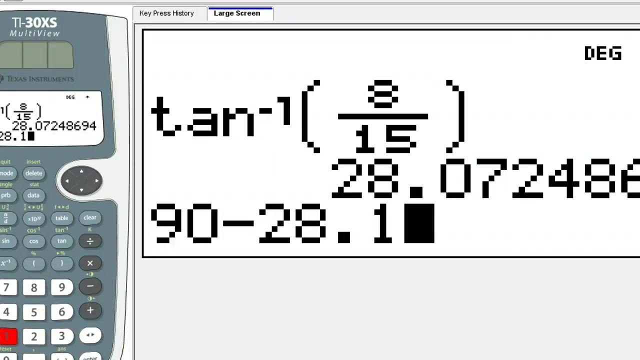 degrees. okay, so that's one angle. all right to find the other angle, we will do 90 minus 28.1,. okay, so 90 minus 28.1 degrees. let's see 90 minus 28.1,. 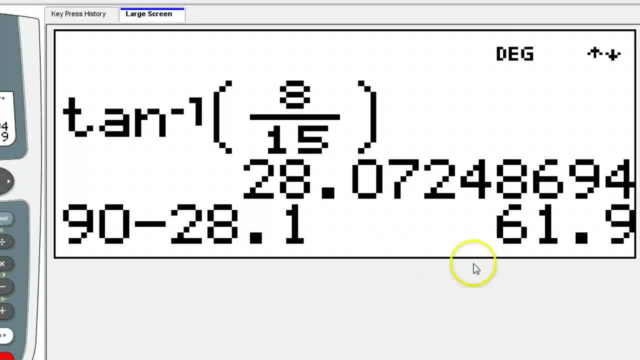 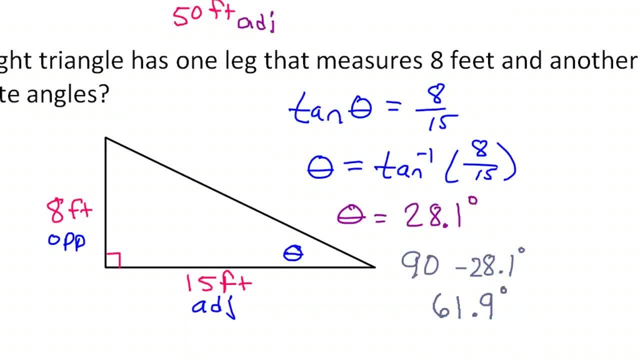 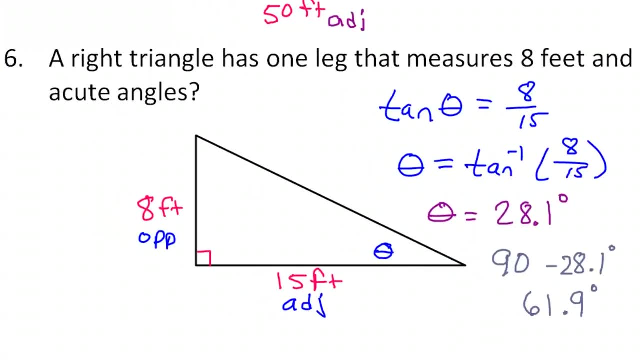 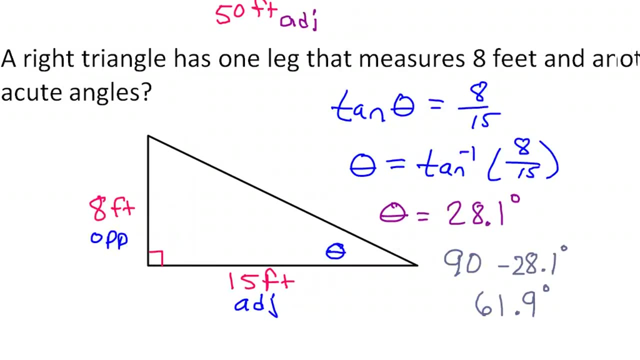 is 61.9,. okay, so that's 61.9 degrees. okay, so that means the two angles. if you put those together for the answer, it's 28.1 degrees and 61.9 degrees. I'll just put it over here. 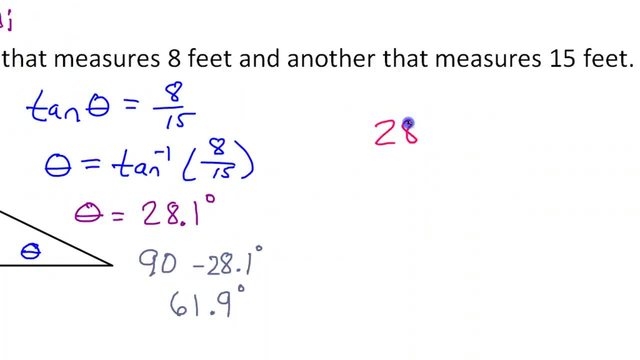 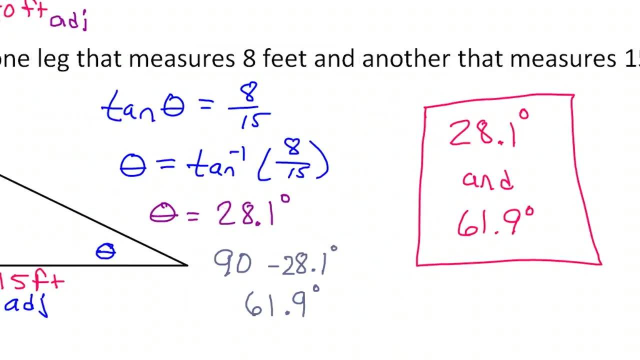 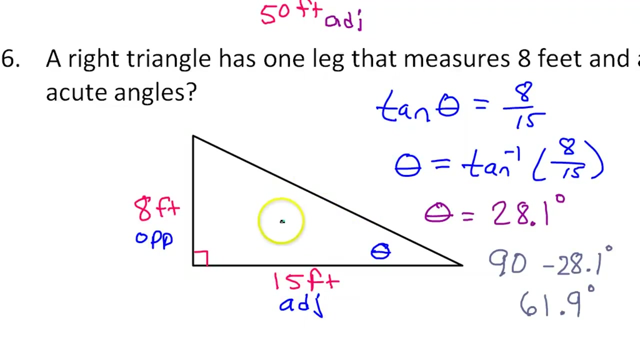 okay, so 28.1 degrees and 61.9 degrees. all right, and that is the end of this lesson. I hope it was helpful. Please make sure you can do each of these problems by yourself, without just copying off the video. I'll see you on the next video. 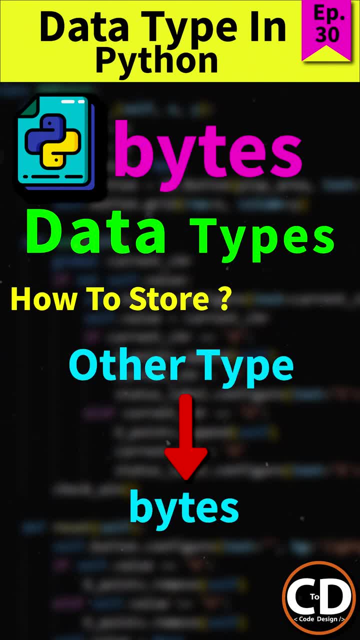 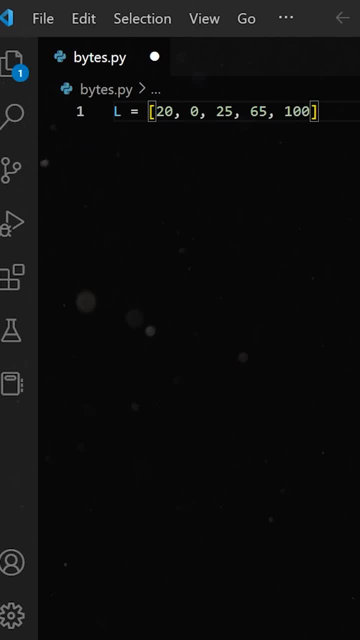 Bytes data type in Python. In last video we discuss about the basic of bytes data type. In this video we will cover the rest of the topic. So, for example, let's create a list and then convert it into the bytes. Now if we print it and check its type, then we can see that it's 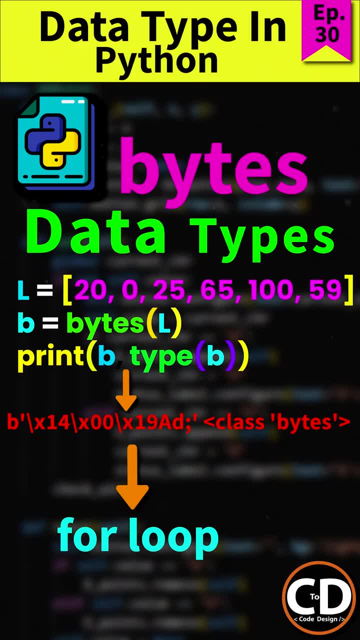 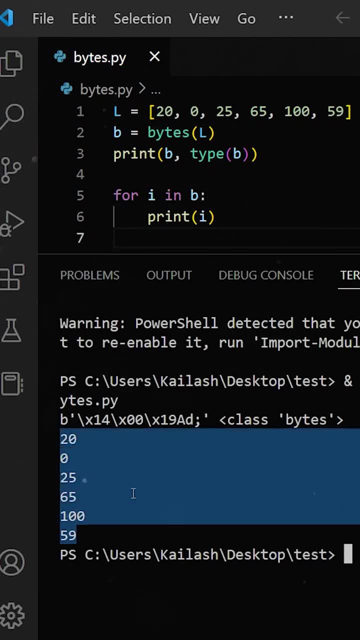 not readable, but the type showing is bytes. So in order to read the data, we have to use the loops. So let's use the for loop for getting all the values of bytes object. So, as you can see, if we use the for loop here, then we can get the values of the bytes data type And as we 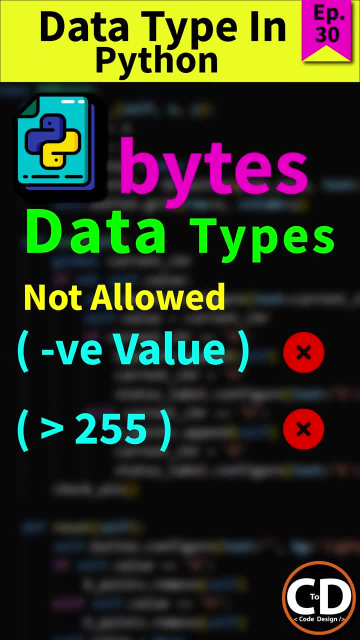 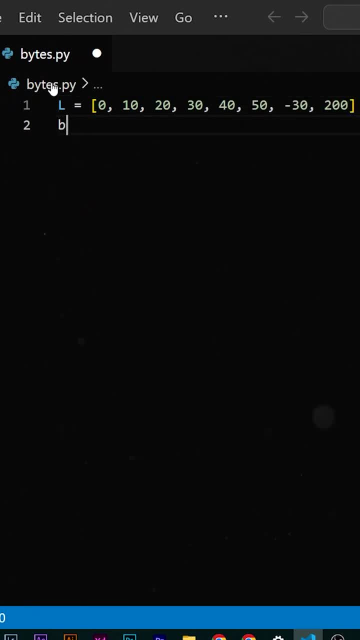 discussed earlier that the bytes data type can only store positive number in range between 0 to 256. So if we create a list and add a negative value in it, then you can see it's showing the value error and also showing that bytes must be in range 0 to 256.. The same will happen if we try. 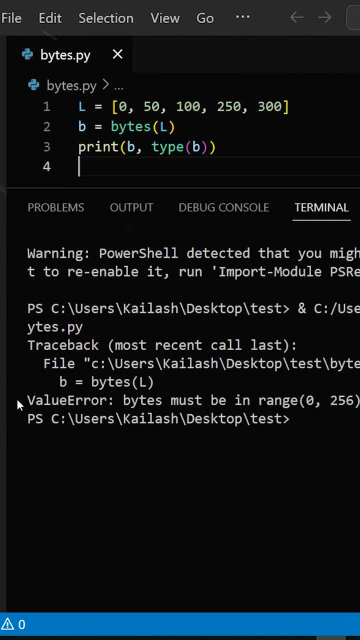 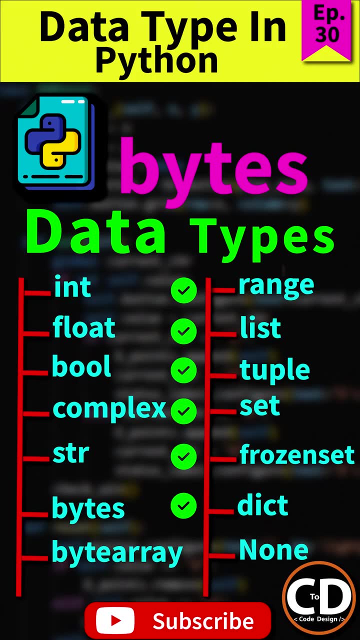 to add a value that is greater than 255, we get value error. And also if we try to add any string value into it, then it will show type error. Thanks for watching. In next video we will discuss the remaining data type. Till then, subscribe to our channel.